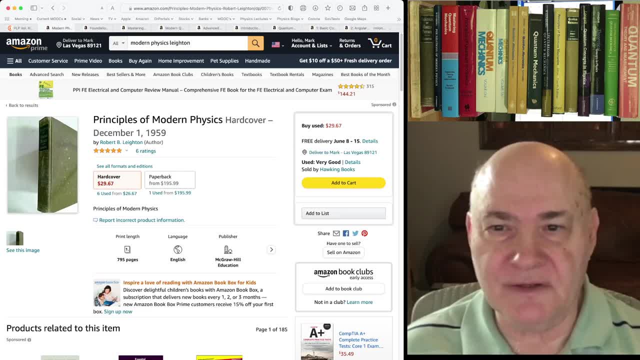 by Leighton, who was at Caltech At that time. it was actually given to seniors But it covers an awful lot of quantum mechanics, where it starts with relativity and then it goes to the Schrodinger equation and atoms, molecules, nuclei and elementary particles And it covers 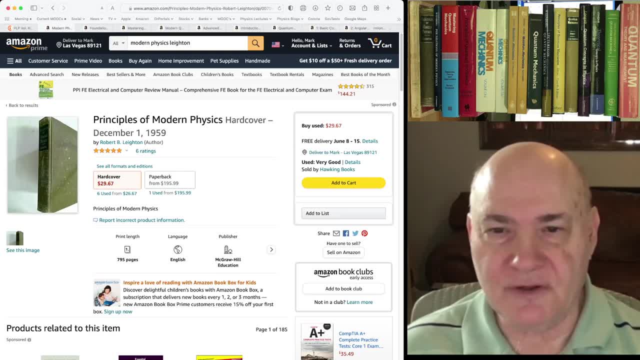 things like x-rays. you know topics that are often ignored nowadays. As we get into, we have to push things earlier and earlier into the curriculum, So this book covers like holes. Now what you need to do as a student is to find an updated. 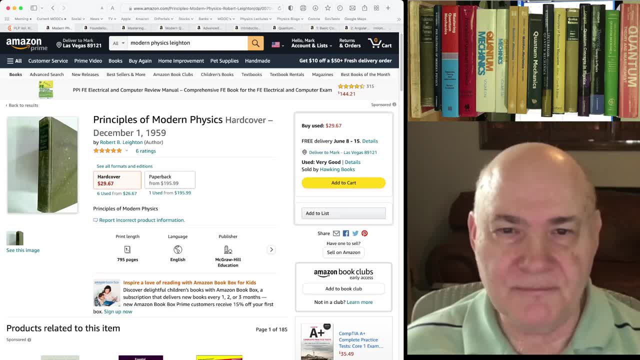 version of this book. There are many modern physics books out there and I haven't looked at them, So find one that's good. that's like a little past freshman level, not much past freshman level- and take a look at it and maybe it can you know, do the holes that a lot of 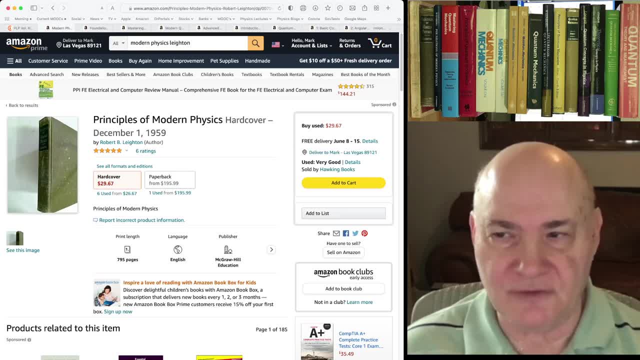 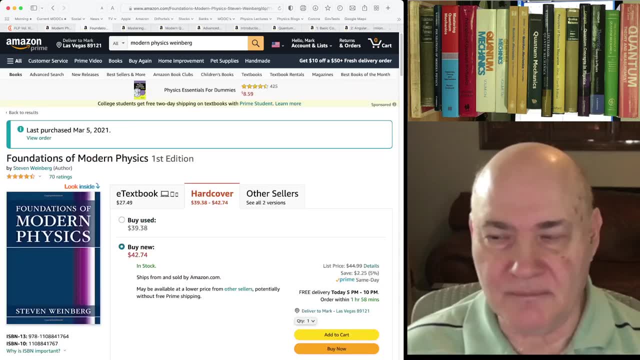 quantum mechanics books don't treat. nowadays, They sort of go past it. Some do, some don't. There is an excellent book on modern physics that was published a couple of years ago by Steven Weinberg, who recently passed away, But this book is a little bit too advanced. 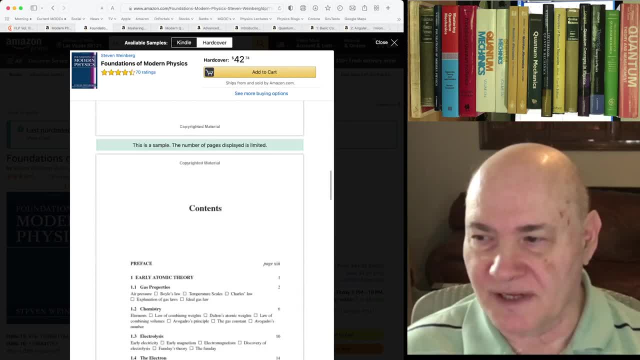 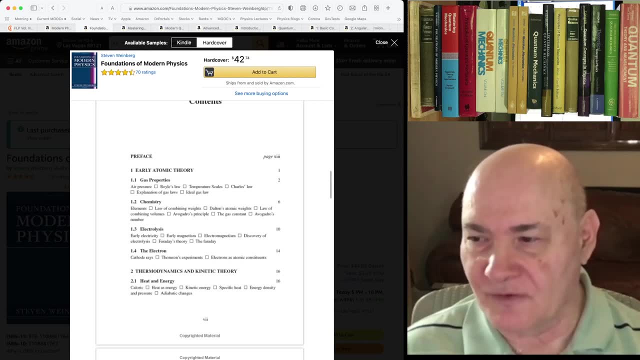 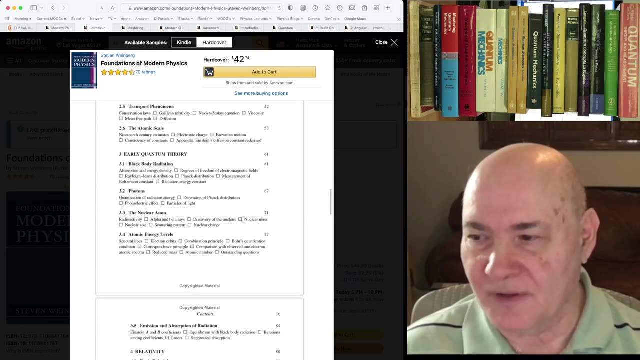 It starts in the beginning. I might have written a review about this book. it starts in the beginning very good with like early atomic theory and how they measured things and thermodynamics and kinetic theory and all of this stuff. But then when it gets and the early quantum theory, but when it gets into 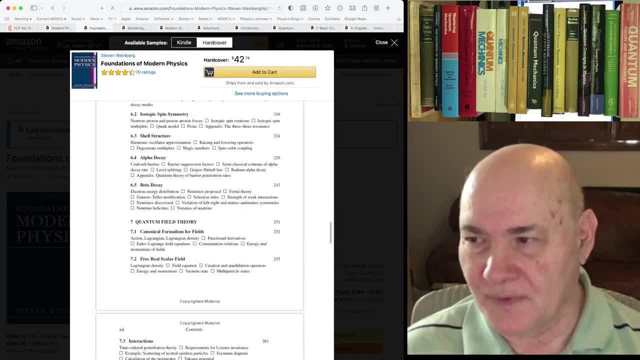 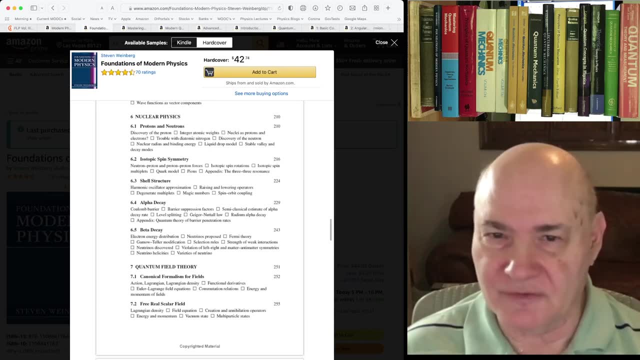 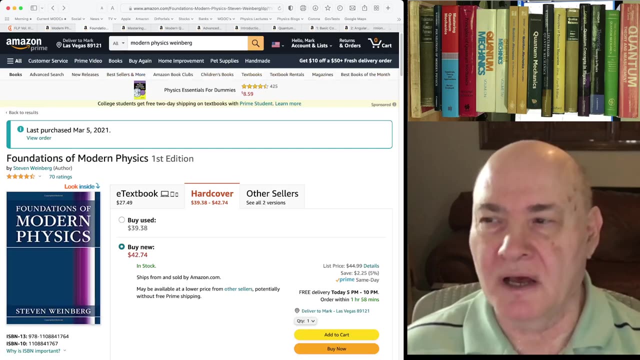 relativity and quantum mechanics and wave nuclear physics and quantum field theory. you really would have a hard time understanding this unless you've already had a quantum mechanics course. So I actually recommend reading this book after you've taken a quantum mechanics course, not before. 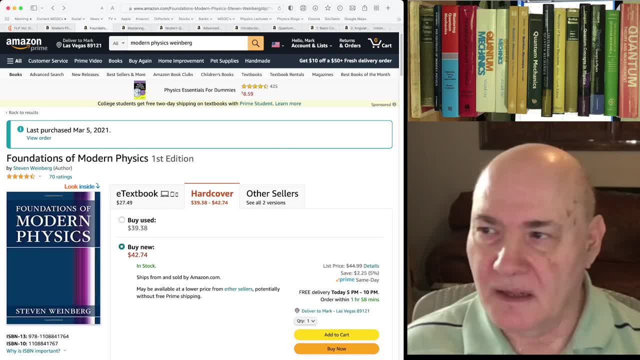 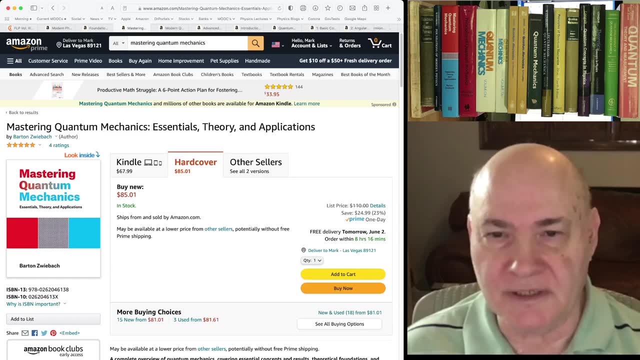 Now, since I made this video, Barton Zybeck's book on Quantum Mechanics has come out, and I recommend this above all other books for a beginning student. The book is based on notes for the three MOOC courses that I was involved in. as in the discussion, 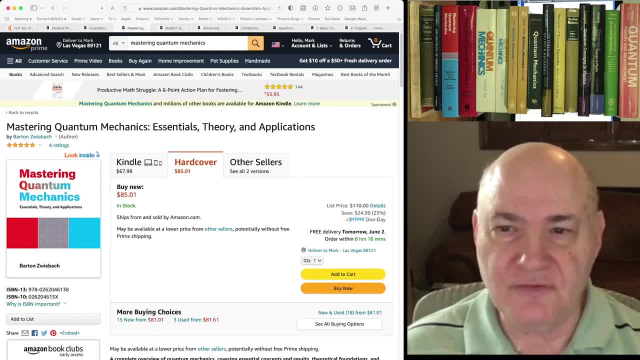 forums and that was run by MIT and edX, And they have video lectures online at MIT, OCW and eventually will be run again on an MIT site, and so it's a great way to get a book that closely tracks a video course with exercises, problems, solutions and exams. 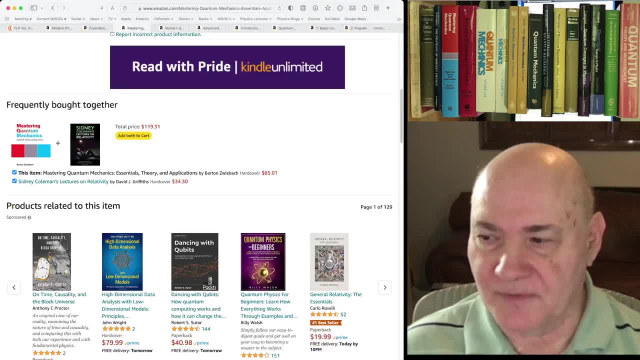 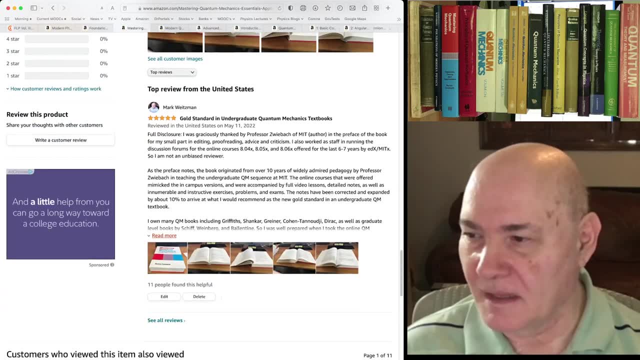 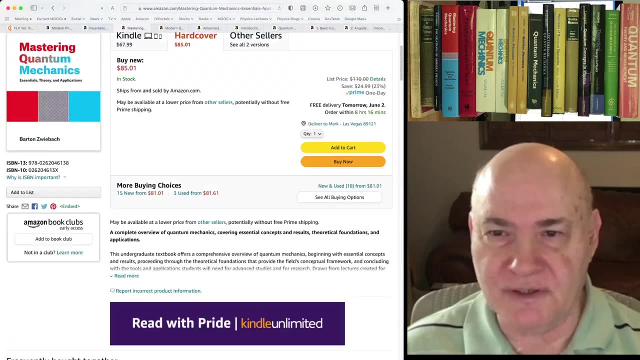 But I wrote a review of this book on Amazon, a very long review. I think I'm still the only review on it, but you can see how long this review goes, so you can read more details about it. What I like about this book is that it's really like three courses in one. 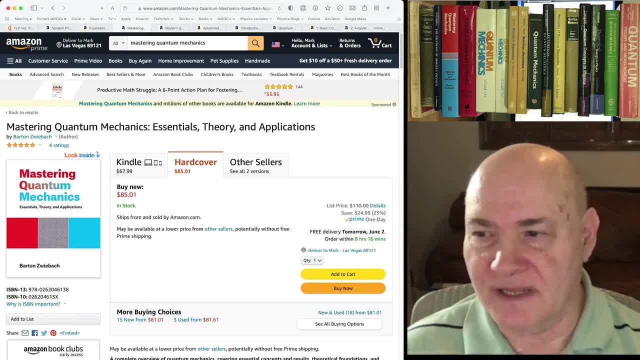 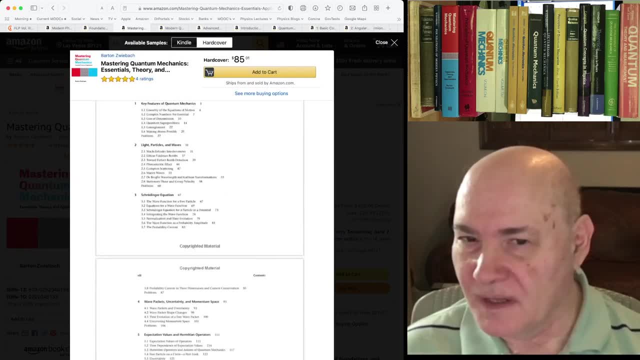 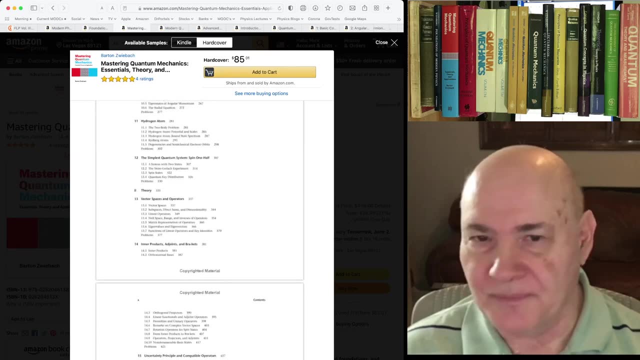 It starts out with what's like a sophomore level course on quantum mechanics and you can look on the table of contents and see that this covers, you know, your basic things on quantum mechanics, up through the hydrogen atom and everything. It finishes with spin. 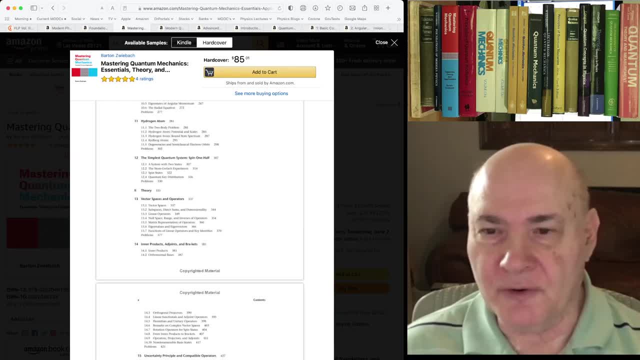 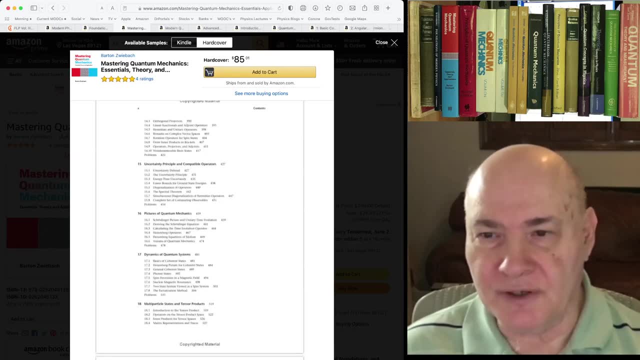 But it doesn't do the theory in detail and it doesn't do perturbation theory and various other advanced topics in detail. Okay, This is in part two. Part two and three are like after you've had an introductory course in quantum mechanics at the sophomore level. it's a rigorous full year course, you know, like given by Caltech. 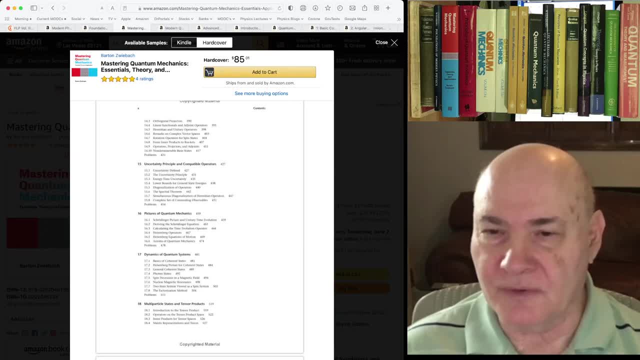 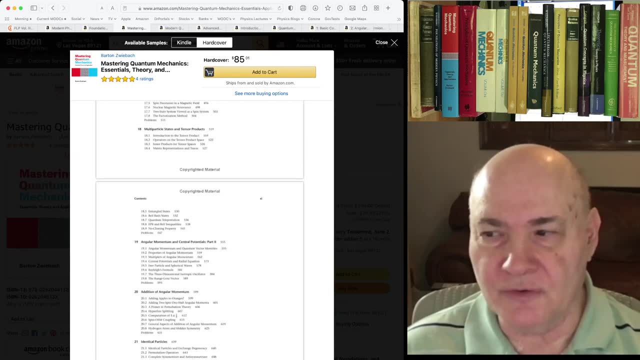 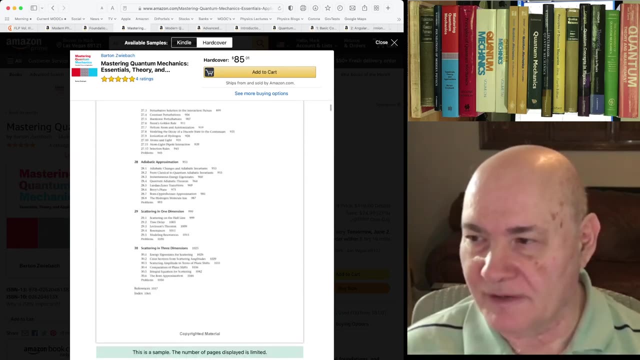 and MIT and other top institutions where they have three semesters on quantum mechanics, And so the theory is given in volume two and some of the applications And then in volume three it covers really advanced material on, like scatter Scattering, the adiabatic approximation WKB. 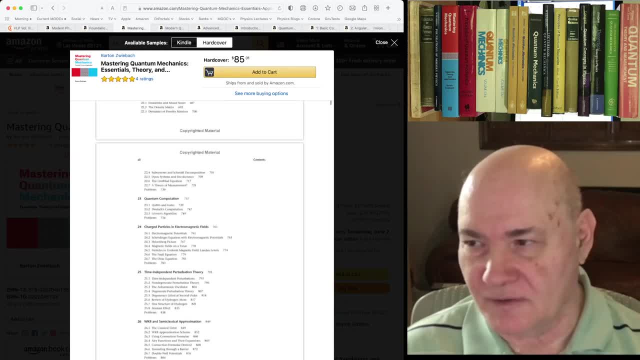 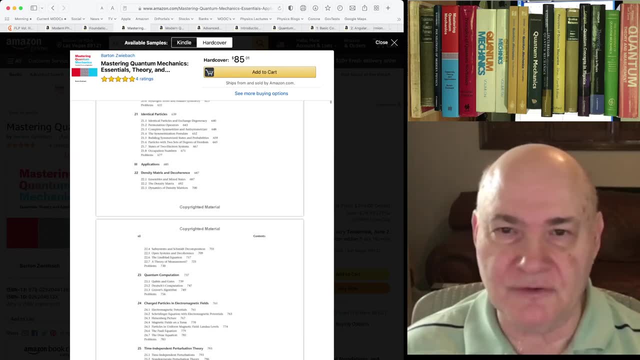 It does perturbation theory like the best I've ever seen. it degenerate perturbation theory And there's a chapter on density matrices and it's thoroughly modern. this book things about Bell's inequalities, quantum computation, cryptographic applications and everything. 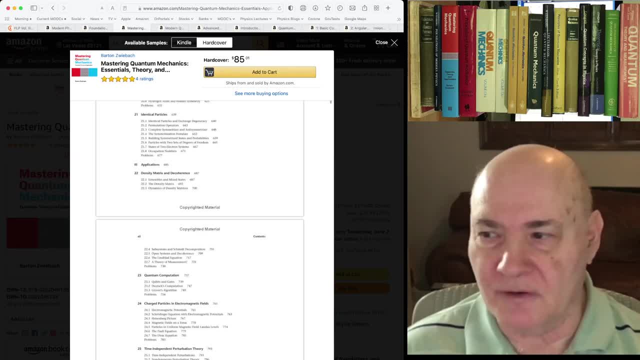 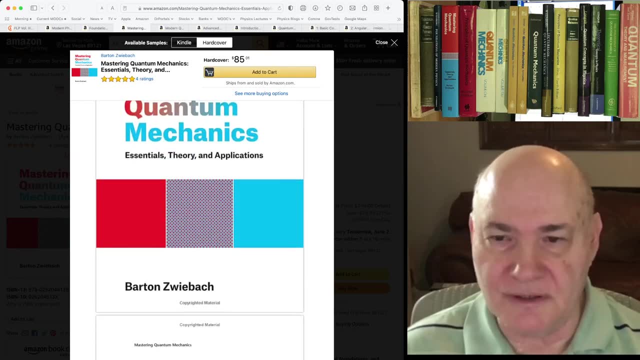 They're all included in this book- the BB84 key protocol, So it's really an updated quantum mechanics book. It's a book that still covers the traditional material. It's a thousand pages long. It's in a sense three books in one, but I highly recommend it. 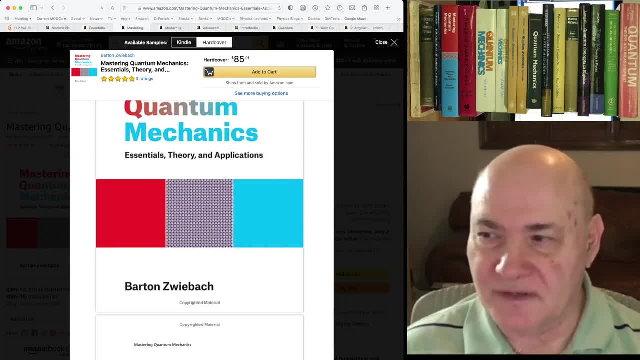 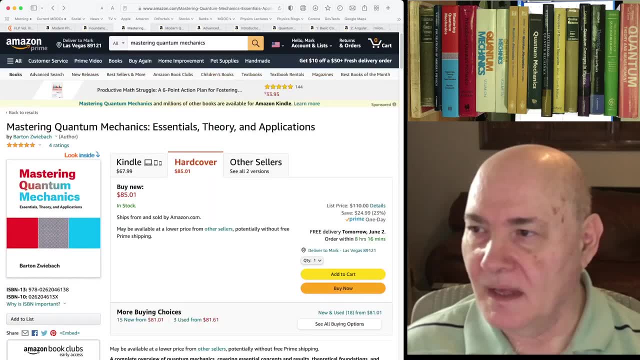 And you can read my review on Amazon. This is definitely. if you want a quantum mechanics book and you're a student, this is the one to start with. One of the main, at least graduate level, quantum mechanics book I should probably. 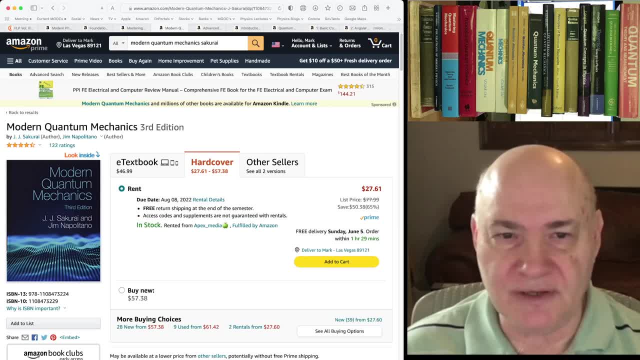 have this later in the thing is Modern Quantum Mechanics by Sakurai. I haven't read this book. It gets very good reviews. I've seen some problems from the book and they're very good. The only thing I can say is that Sakurai died before the book was completed, so it's not. 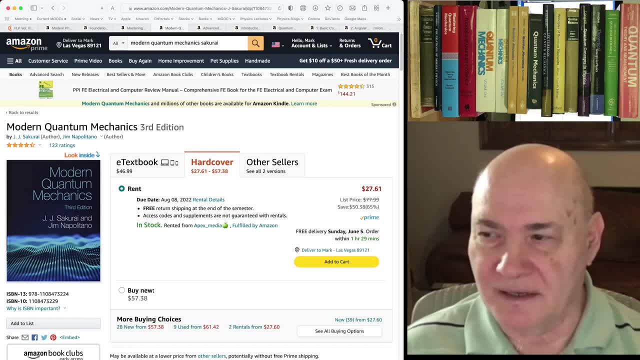 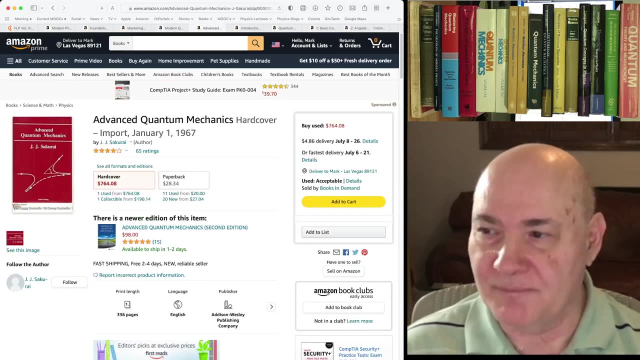 really written completely by Sakurai And it seems to be more of an outline of a book than a detailed presentation, like some other graduate level quantum mechanics books. But anyway, this is used in many places and you shouldn't confuse this with a great book. 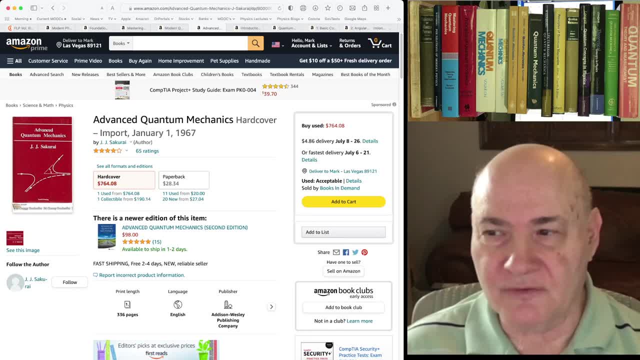 that Sakurai wrote. He wrote all by himself- called Advanced Quantum Mechanics, which is really extending quantum mechanics to the relativistic domain and also quantum field theory. So this is an excellent book to read before you begin your quantum field theory studies. 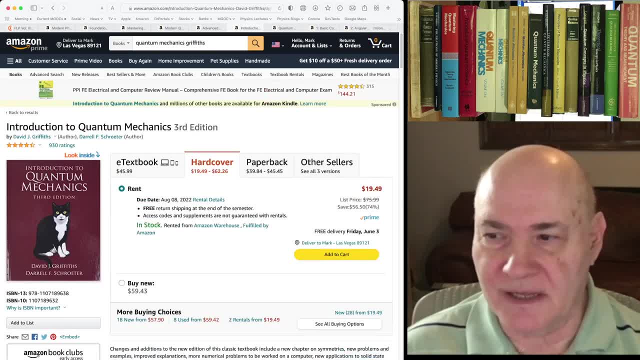 Other standard. this is probably the most loved book on quantum mechanics by Griffiths. It's an excellent book. I have read it. The main problem is it doesn't go deep enough. It doesn't go deep enough. It talks about Dirac bracket notation, but then it doesn't use it. 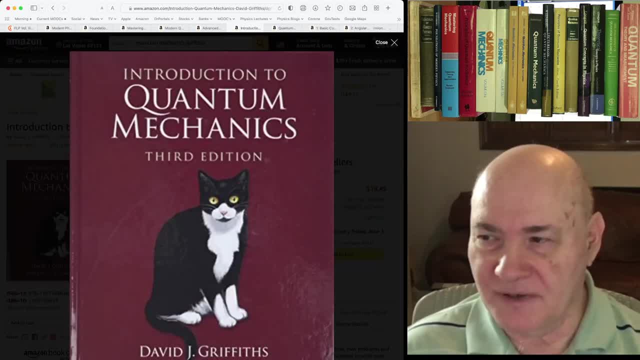 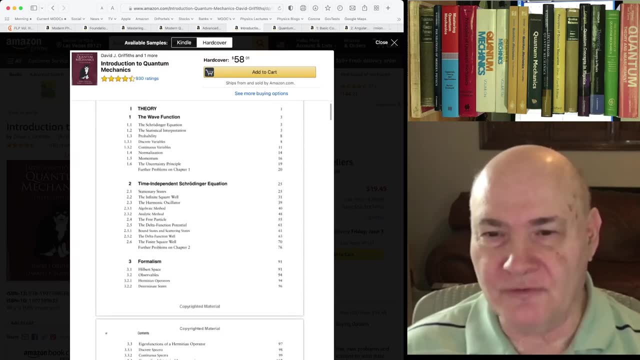 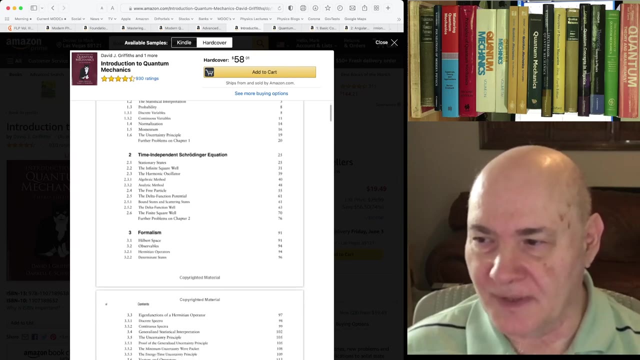 It's mostly a wave function book, but it's got some excellent chapters and he writes very well. And the other thing is that he just presents the Schrodinger equation on page one. He doesn't even attempt to give a motivation for it or a derivation or something. 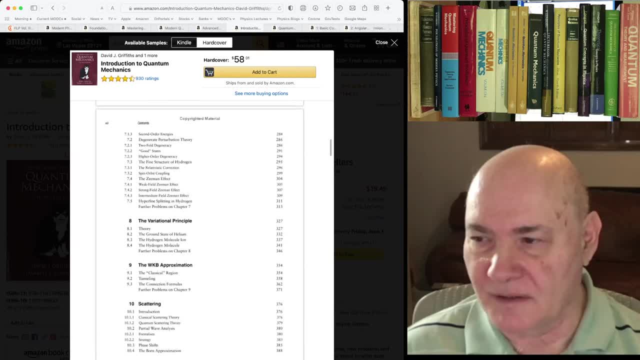 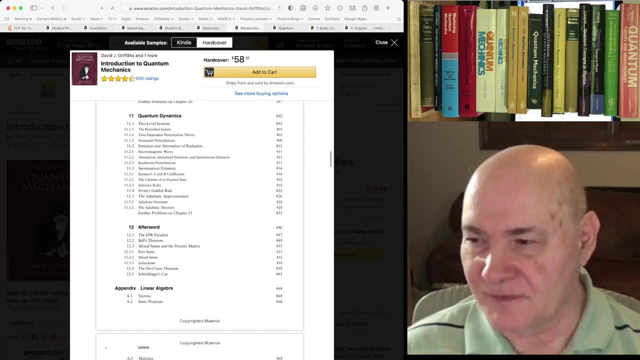 But there's a lot of things in this book and students seem to like it. Usually when students like a book a lot, it means it's easy and I suspect this book is relatively easy. I think the third edition has been updated a little bit to EPR, paradox and various. 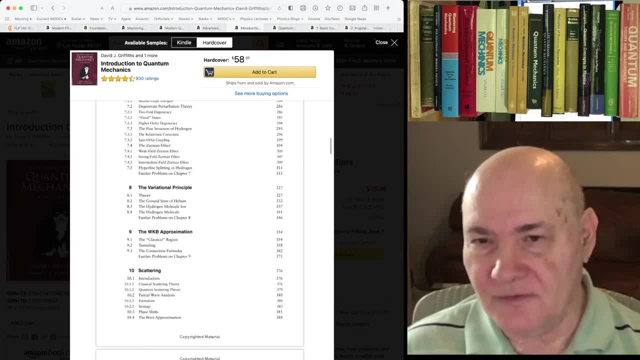 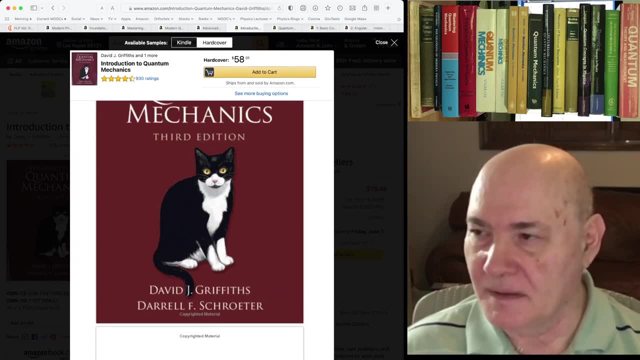 other things, mixed states. So this is an excellent book and if you're using it in a course or if you want to read it, I recommend it. The second most popular quantum mechanics book is the Schrodinger equation. It's a very interesting book. 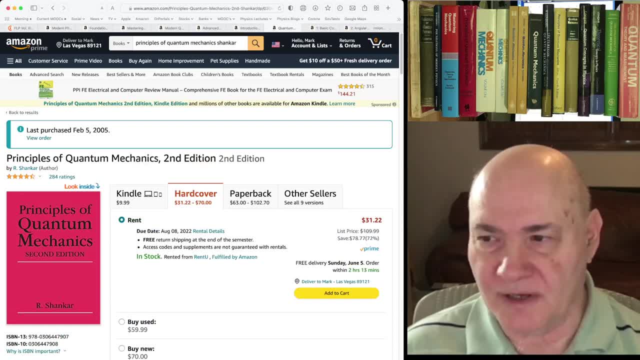 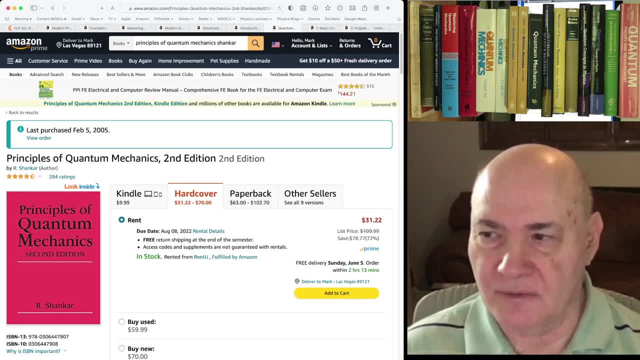 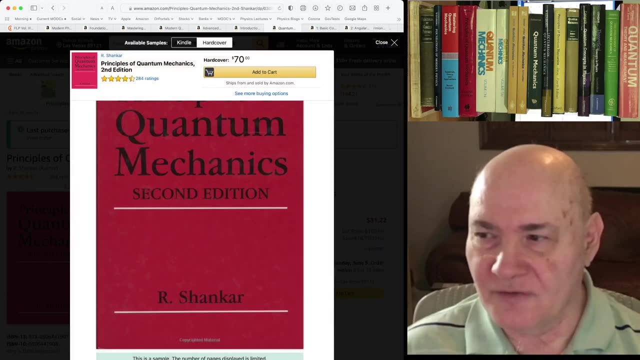 It's a very interesting book. It's a book by Shankar. This book is Principles of Quantum Mechanics. It's an interesting textbook. The author is like his main research area has to do with path integrals and condensed matter and he's got several chapters. you know, like mastering quantum mechanics doesn't. 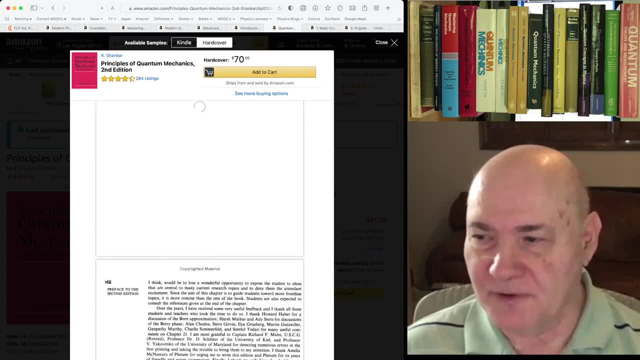 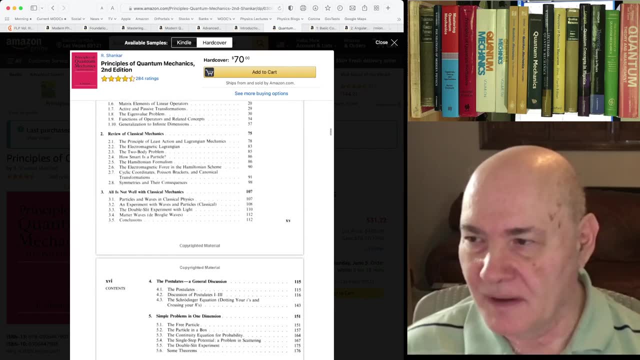 treat the path integral. It leaves it to graduate level. But this book treats the path integral in several places In addition to a long final chapter. But he's got an excellent, very good linear algebra review for about 60 pages at the start. 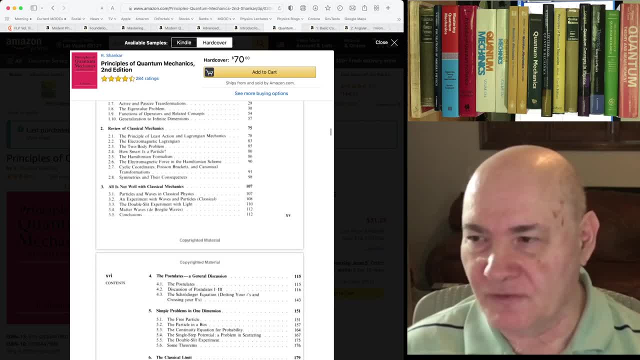 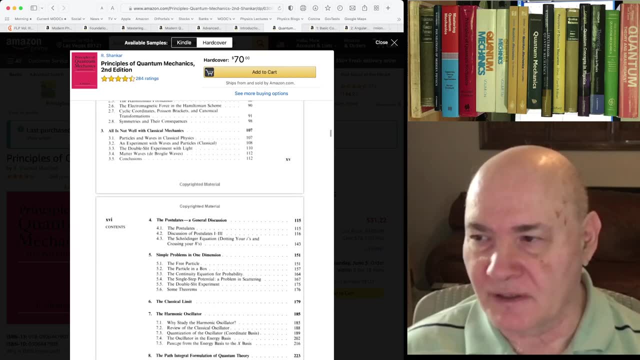 of the book, which is, you know, fairly good, And he reviews classical mechanics. So if your physics is a little weak and your mathematics is a little weak, this is a really good book for reviewing a lot of stuff, And then he has several chapters. 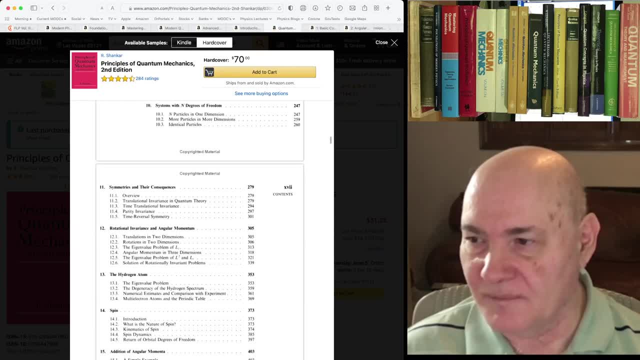 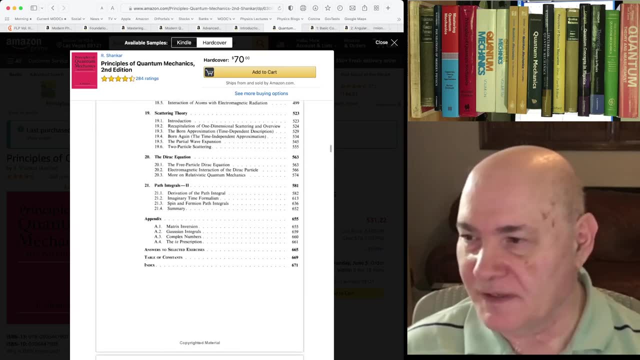 He starts, he has a chapter 8 on the path integral formulation and then at the end of the book He has a very long chapter path integrals, like about 70 pages on. you know imaginary time, formalism, fermion and spins and various other things. 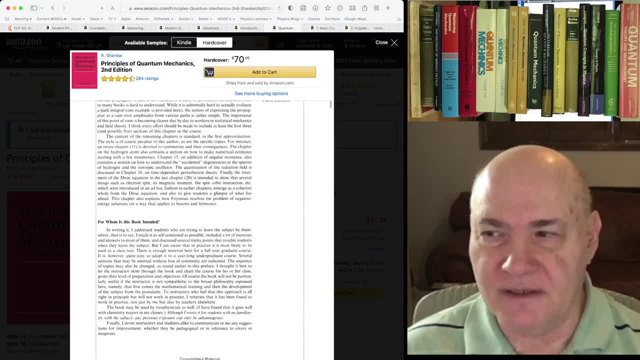 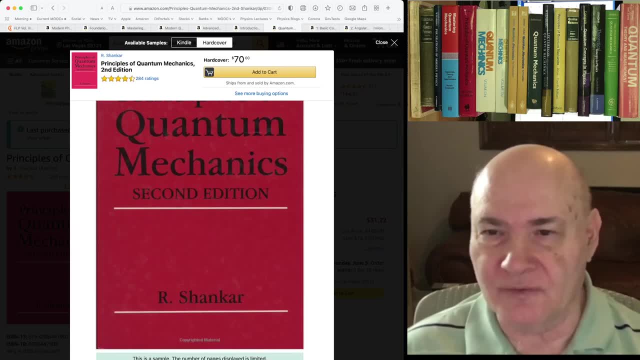 So I like Shankar a lot. I think the book is a little weak in the problems. He doesn't have enough of them and he interrupts the chapter's flows with like exercises and derivations which aren't really too good, and he definitely needs more problems in the 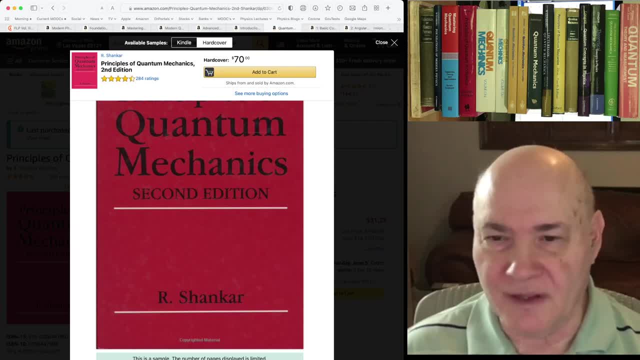 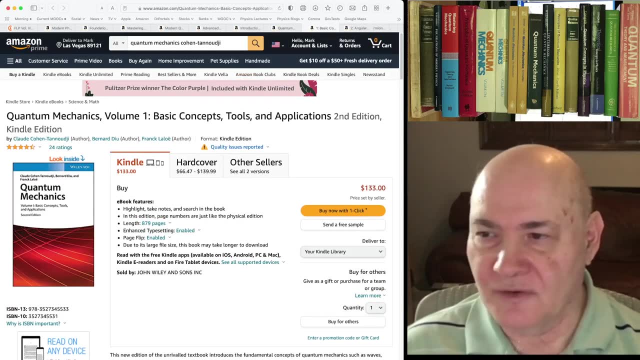 book. So that's the weakness of this book. in my opinion, The strength is that final chapter on path integrals. The next book is more of a reference book. It's been a long time reference by Claude Cohen-Tannoudji. It used to be two volumes and 1,500 pages but after about 40 years they finally came. 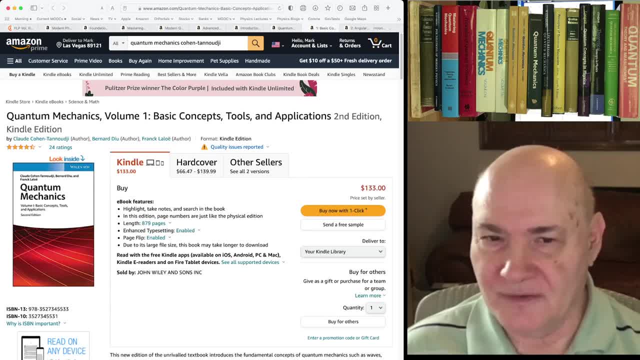 out with the second edition. So there's the second edition And I don't think too much has been updated in the first edition. The volume one is the basic concepts and tools. These books are expensive. That's well, maybe not that expensive: 66 to 140.. 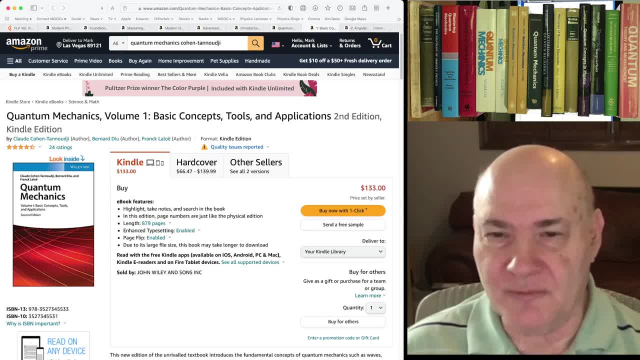 But if you want a textbook that does like the harmonic oscillator in one, two, three dimensions, in rectangular, spherical and parabolical, this is your book. It's really a reference book. It sort of does everything In every different way. 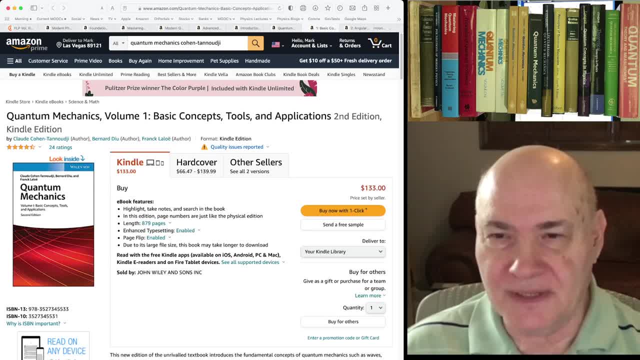 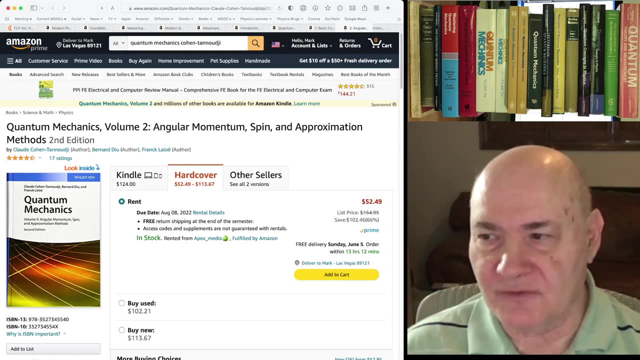 It's written in a little bit like the French style, a little not that exciting, But it stood the time as a reference book for undergraduate and graduate level books on quantum mechanics. And now the second volume treats angular momentum, spin and approximation methods. 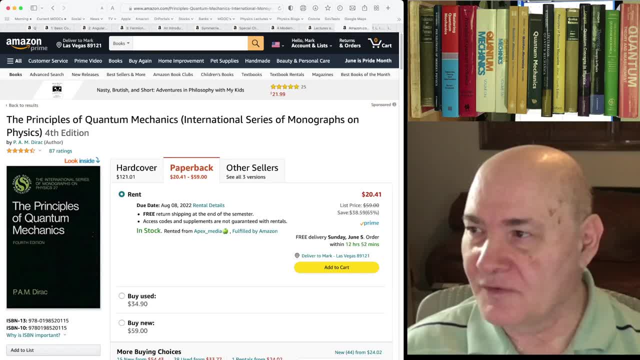 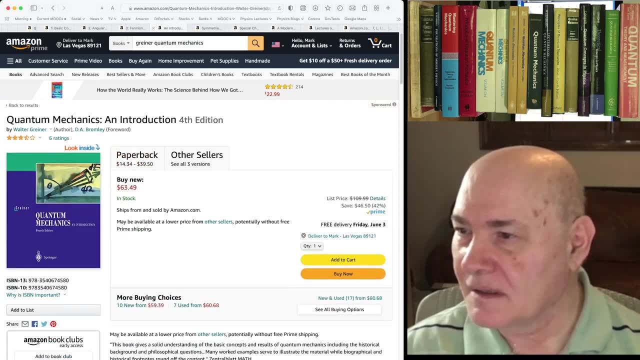 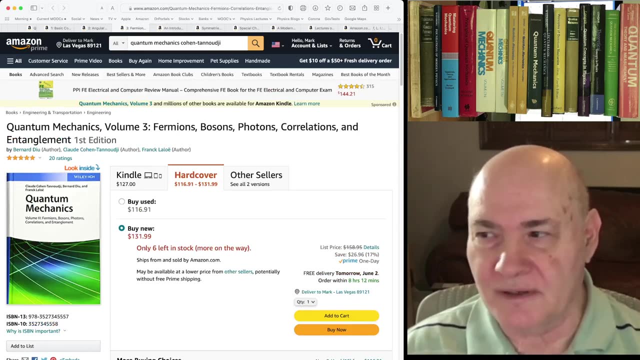 And then there's this new third volume, which looks really interesting. Oops, I got it, Sorry, Where did I go? Okay, This is the volume three of Cohen Intuity. They added a whole new problem on fermions: photons, photons. this is really a condensed. 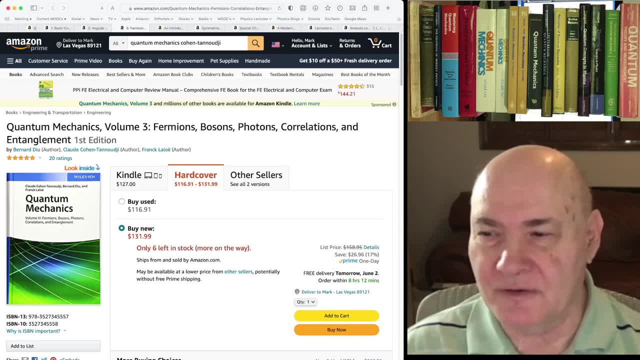 matter and entanglement. So this is a little bit beyond your quantum mechanics course, but it has a lot of interesting things in here. It's more of a condensed matter. Now for graduate level text. oh, two other textbooks I want to mention is Walter Greener. 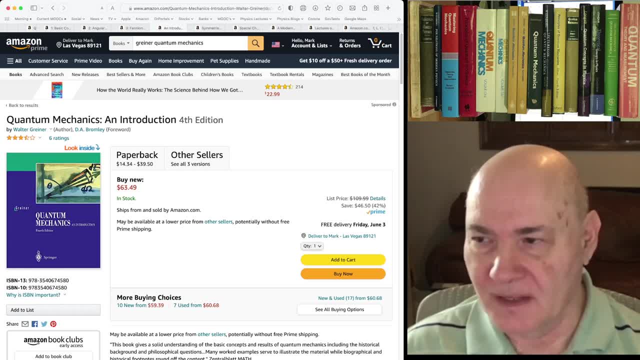 has a whole theoretical thing And he has a whole physics series starting with quantum mechanics and going through all the way through the standard model. There's probably about 10 to 15 volumes in the series And they're all sort of like workbook series. 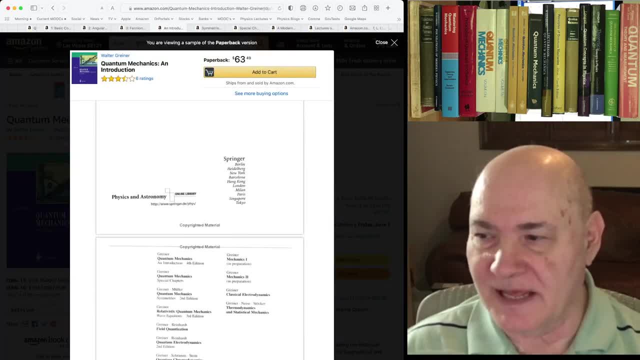 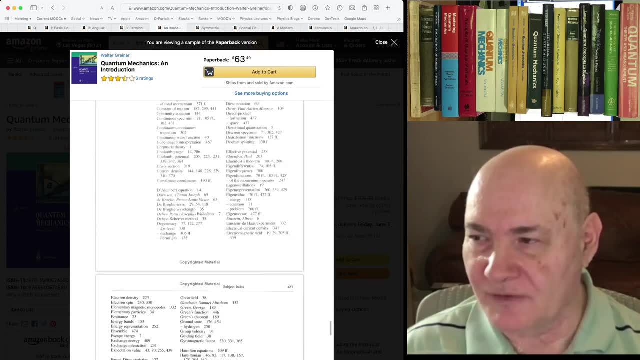 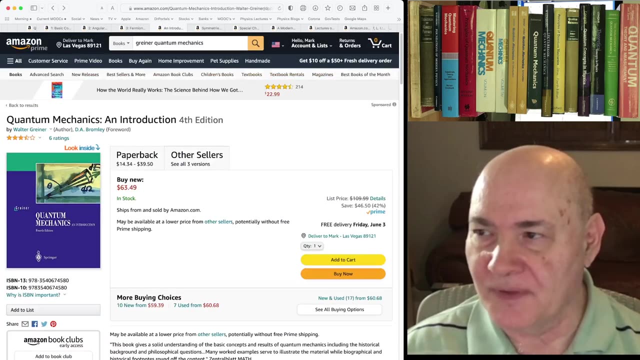 I really like them because he has a lot of detailed calculations and examples that you just don't see anywhere else. You know everywhere else. they sort of like shorten the presentation, But here's a couple. But he gives a long presentation and so this volume, the first volume, Introduction, is 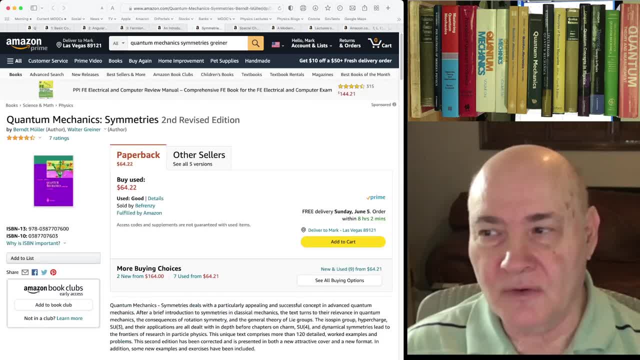 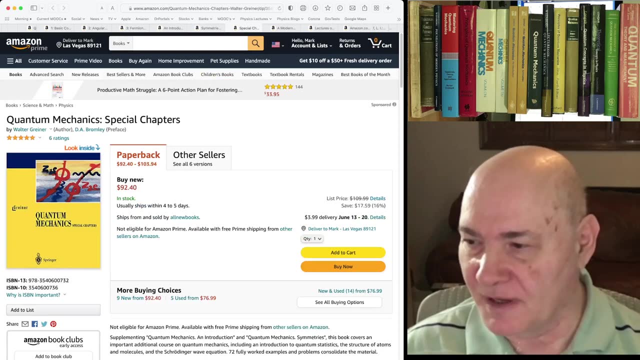 very good, But he also has two excellent follow-up books. Quantum Mechanical Symmetries is more on group theory and I'll have this in my group theory playlist. And then he's got another follow-up book on special chapters where he treats all kinds. 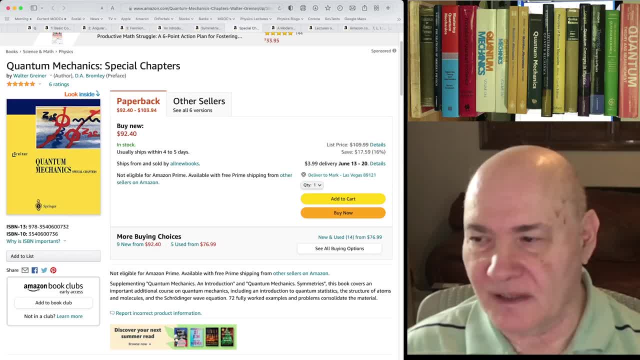 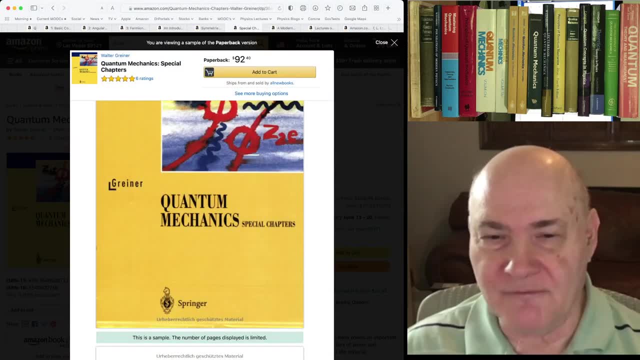 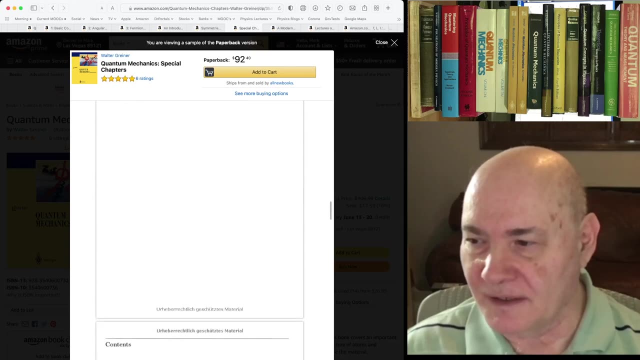 of things on quantum statistics, structure of atoms and molecules and everything. Again he's got like 72 fully worked out examples and problems. So this book doesn't have really like problems. it works them out and solves them for you And it's very detailed calculations and I sort of really like learning from his books. 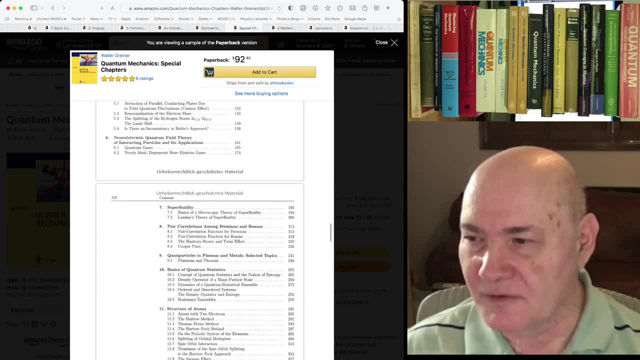 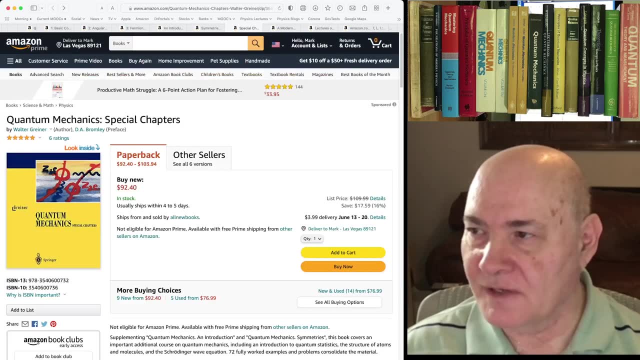 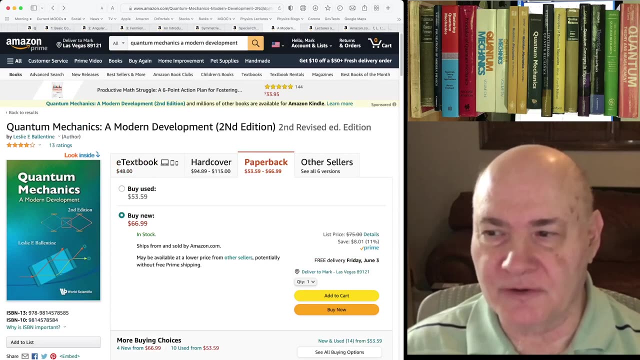 It's not that great as a reference, but it is really good to learn from them and these special topics are very good. Okay, So that's Greener's Like Workbook series. Now, in terms of graduate level quantum mechanics books, this is my favorite one: Quantum Mechanics. 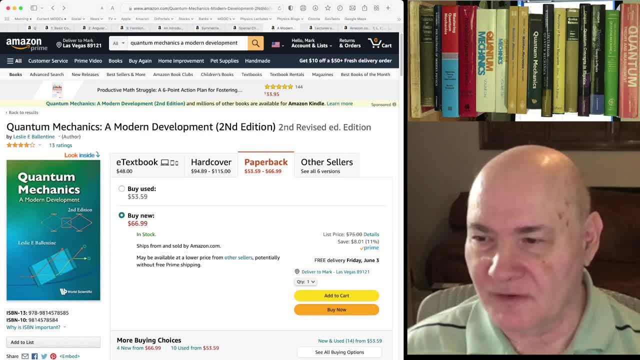 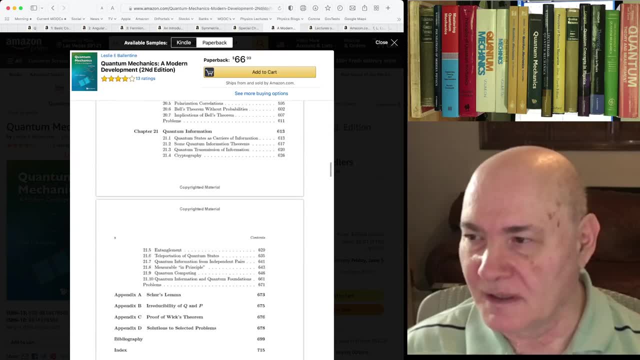 by Ballantyne. Get the latest revised edition, the second revised edition. He added a whole new chapter on like 70 pages on quantum information. But it's a really excellent book. he has a whole chapter on Bell's Theorem as well. 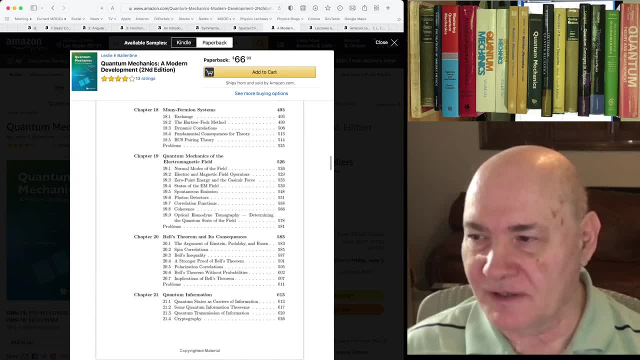 But what I really like is chapter 19.. Chapter 19, Quantum Mechanics on the Electromagnetic Field. It's not the usual quantum field theory treatment. It's a non-relativistic treatment of photons and correlation functions and coherence things you take in a quantum optics course. 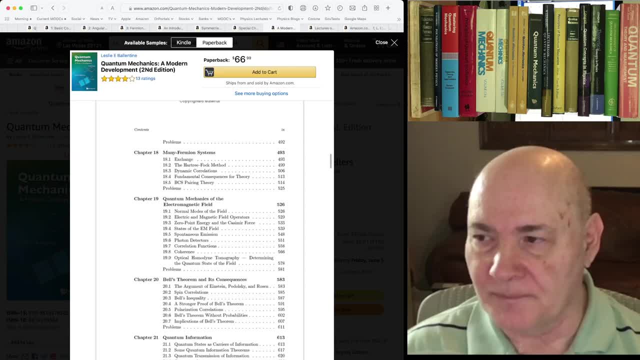 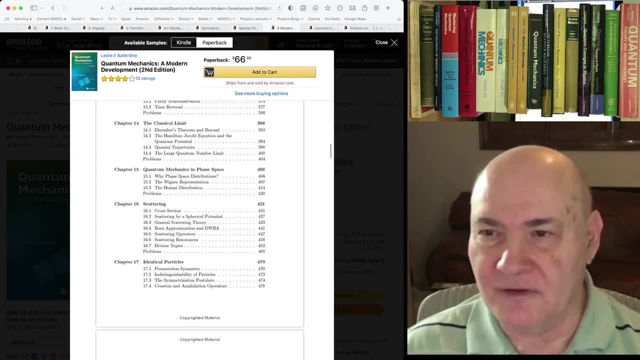 And he has a similar chapter on many fermion systems as well. So the treatment in here is sort of advanced, not too advanced. it's not functional analysis writ large, But he covers a lot of things. He talks about quantum mechanics, on the electromagnetic field. 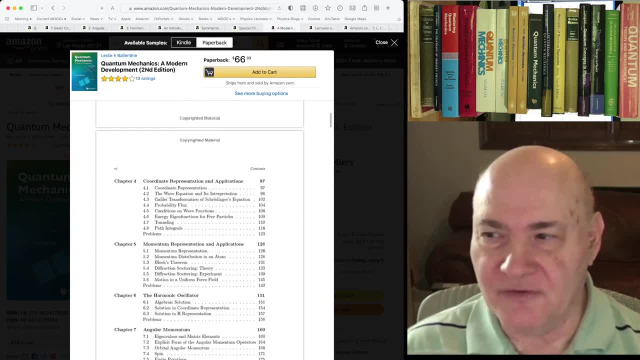 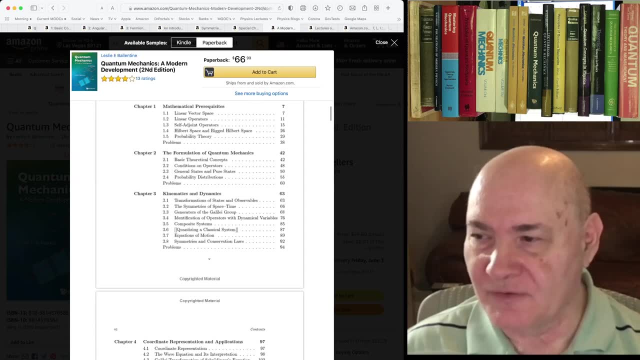 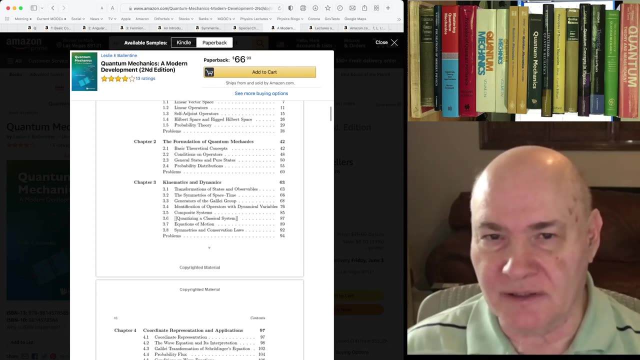 He covers a lot of things that you don't cover: the edge cases, the exceptions, things that sort of get neglected, like transformations on kinematics for the Galilean transformation, non-relativistic quantum mechanics, Things like that he does really really well. 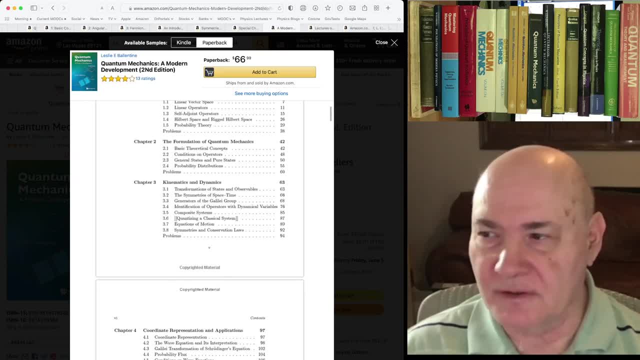 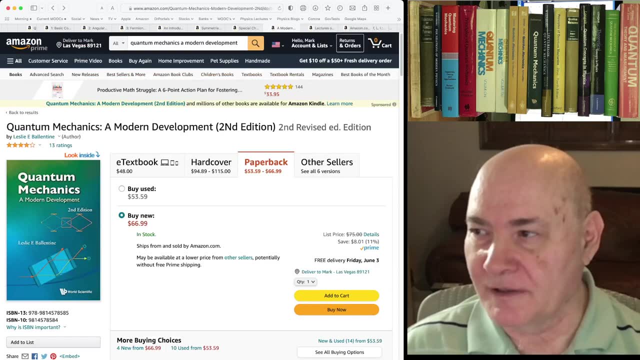 So as a graduate level quantum mechanics book it's not too long. it's about 600 pages, And this is where I would start. Now there's another really excellent chapter on quantum mechanics, Another really excellent graduate level quantum mechanics book, which is Weinberg's book. 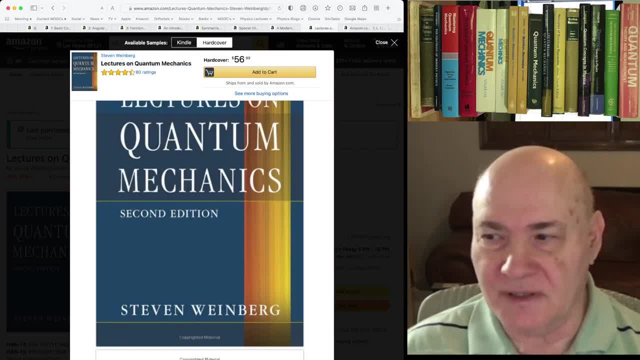 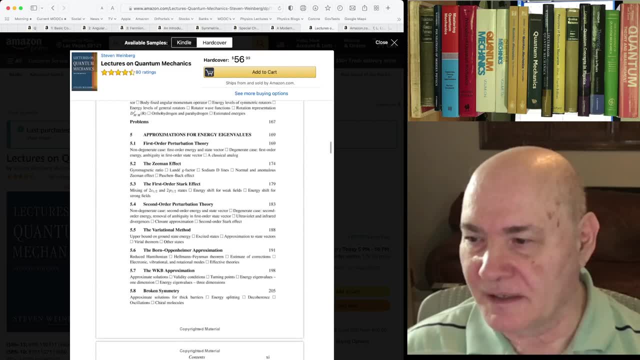 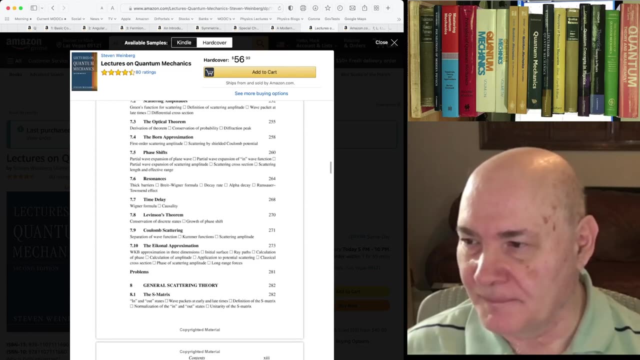 And to me Weinberg's book is like orthogonal to Ballantyne's book in the sense that he treats a lot of topics that aren't treated anywhere else. For instance, he's got a treatment of the Eichenal approximation, and really he does. 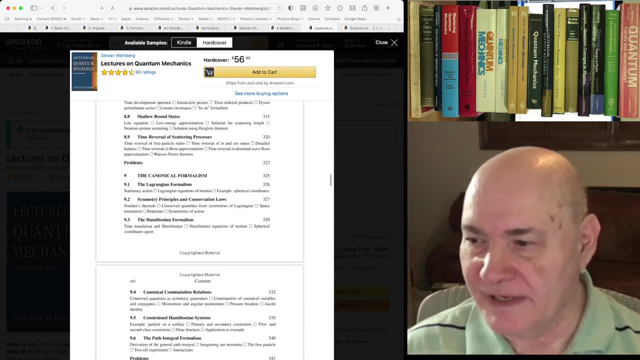 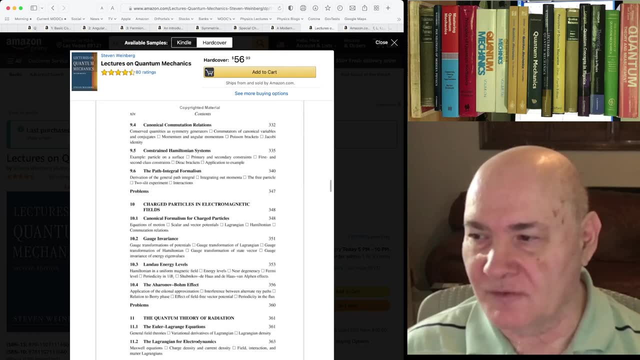 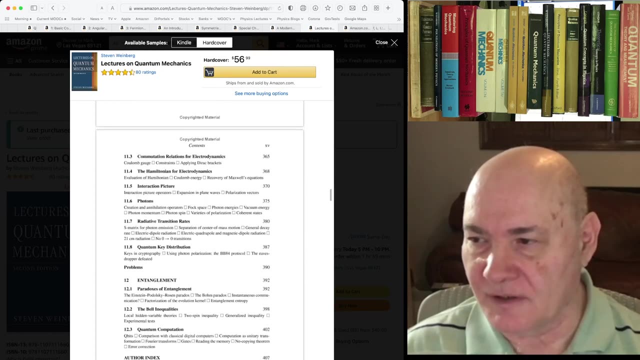 the canonical formulism. He does the canonical formulism, Quantization with constraints. No other book does constrained Hamiltonian systems and everything. So that's where he's really strong and he does a whole quantization like a non-relativistic quantization of charged particles in electromagnetic fields and the quantum theory of radiation. 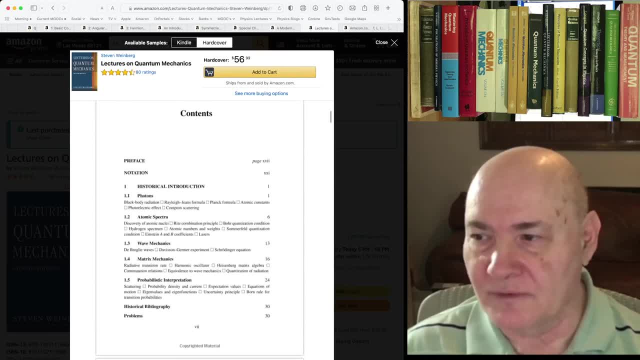 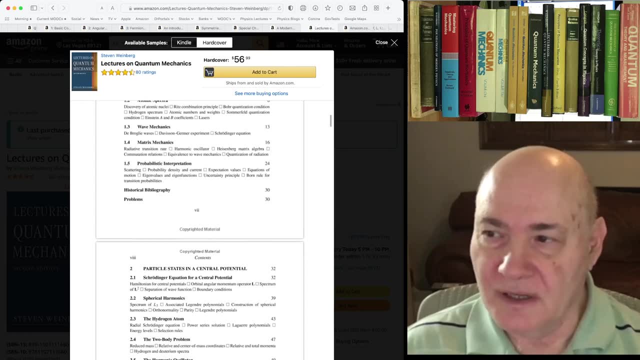 He has a very good first chapter, as Weinberg does in almost all of his books: historical introduction, so you can see where quantum mechanics came from and everything. So, together with Ballantyne, I would say these are the two books that are going to. 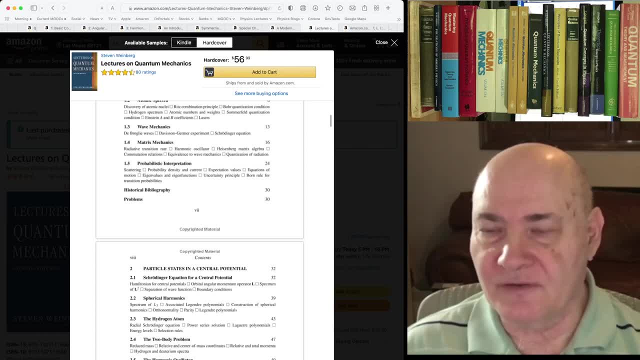 be published in the future. The two premium and he has a lot of excellent problems in the book, although they're often one-sentence type problems and they're difficult. But he, together with Ballantyne- these are the probably if you're on the quantum graduate- 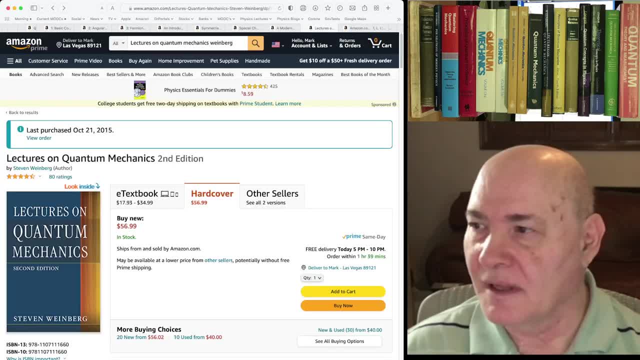 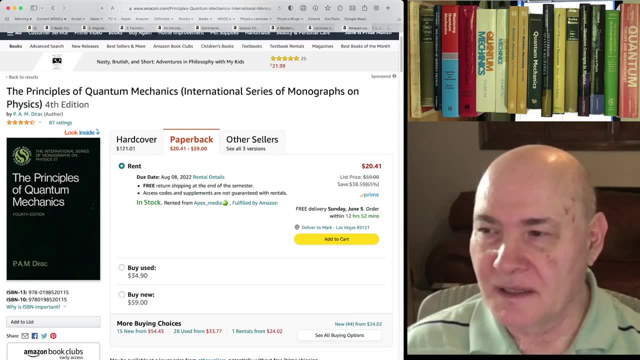 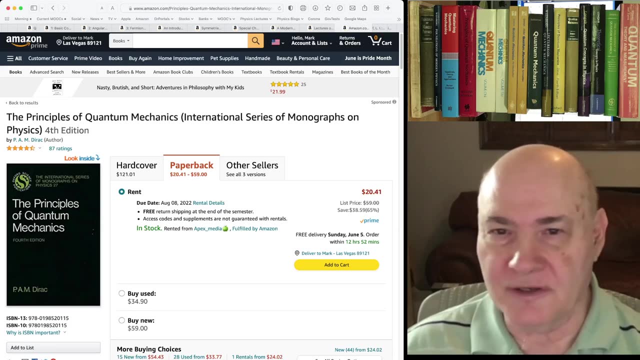 level. these are the quantum mechanics books that you probably should start with. Okay, which one is this? Okay, Anybody who reads any quantum mechanics books should have. You should eventually, at some point, study Dirac's book, the fourth edition, on the Principles. 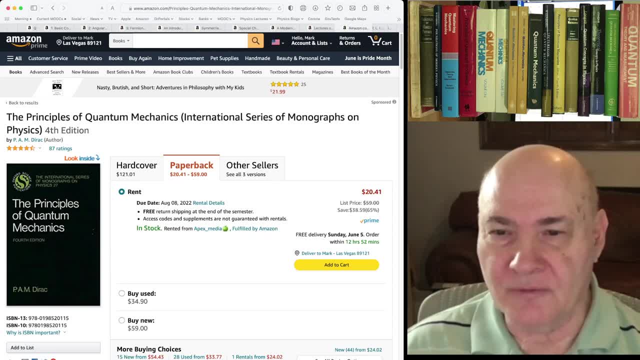 of Quantum Mechanics. It's a really nice read and it will certainly review quantum mechanics but you'll also see how probably the premier founder, the guy who sort of organized the early developments, and Schrodinger and Heisenberg and Pauli- these guys were all involved. 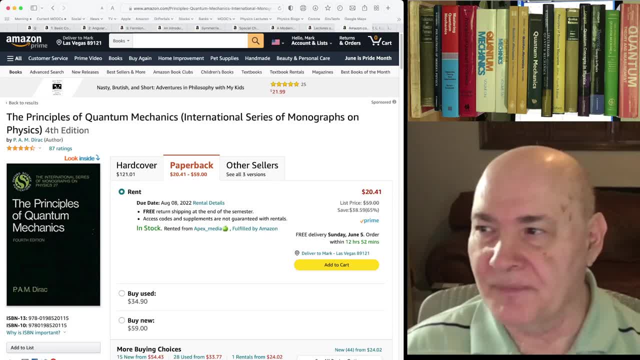 But Dirac sort of invented the language and put it all together as well as coming up with the relativism. It's a very simplistic equation, and with the start of quantum fields as well. So I highly recommend you read Dirac's book on quantum mechanics. 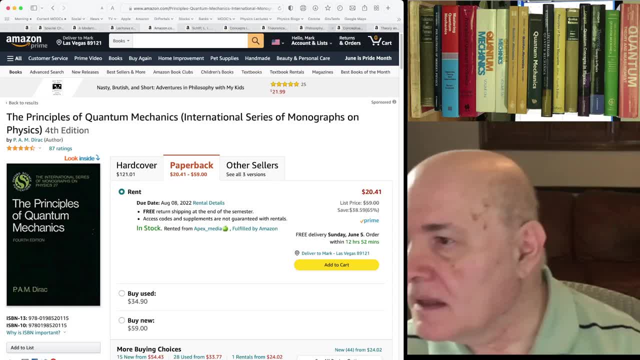 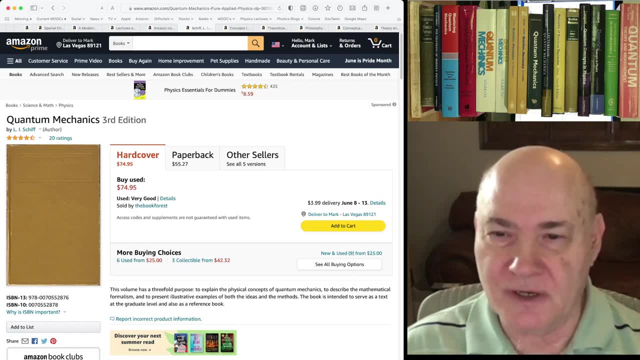 Now, okay, This is an old book. I put this up here. This is one of my favorite books on quantum mechanics. It was by Schiff. It's a classic book. It used to be the standard him, along with Mertzbacher. 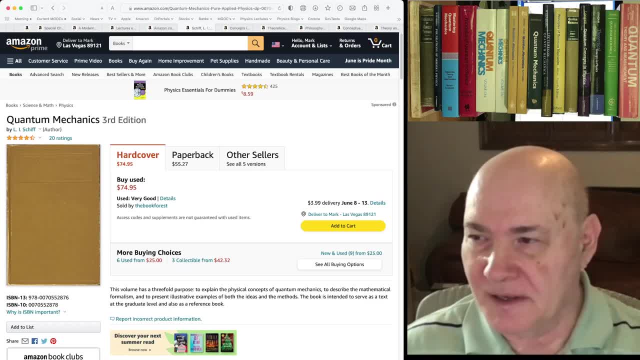 I liked his book to Mertzbacher's book, But you know there's still some interesting things in here that you won't find elsewhere. And if you're looking for an old-fashioned straightforward quantum mechanics book- that sort of came out of Oppenheimer's lectures and everything- read Schiff, or at least look. 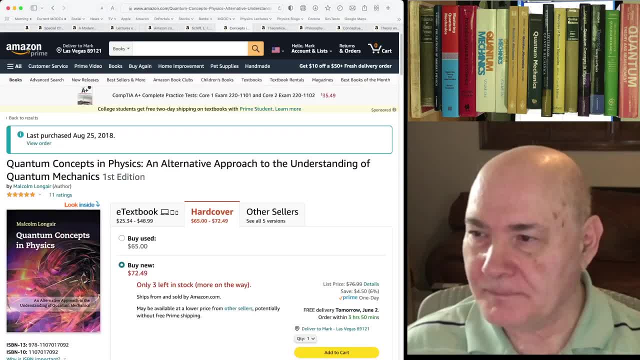 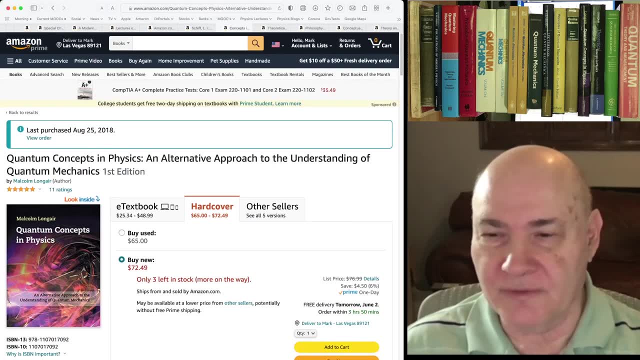 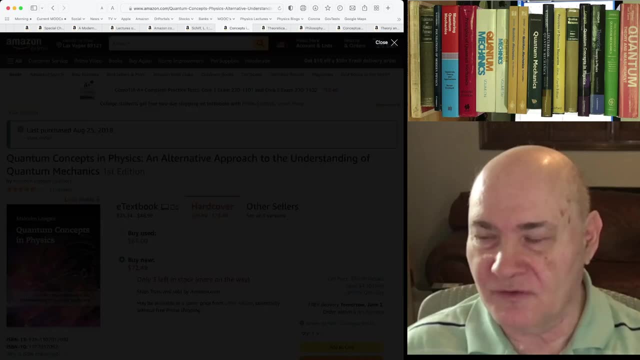 at it. And now, having gone through all these quantum mechanics textbooks, I want to get to the history and philosophy, Okay, Okay. So Schiff, he has a great book, Quantum Concepts in Physics, where he just discusses the whole historical development. 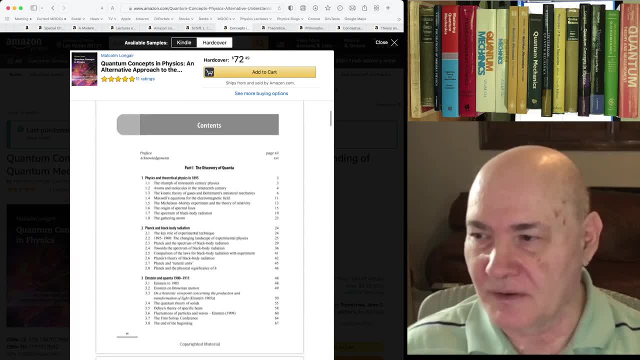 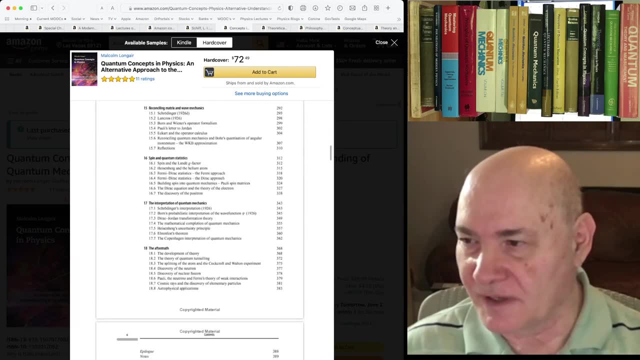 There are several books like this. He does an excellent job. you know equations and everything going from quanta, black body, quantum mechanics and everything, And so, instead of reading the early papers, which are pretty hard to read if you're a 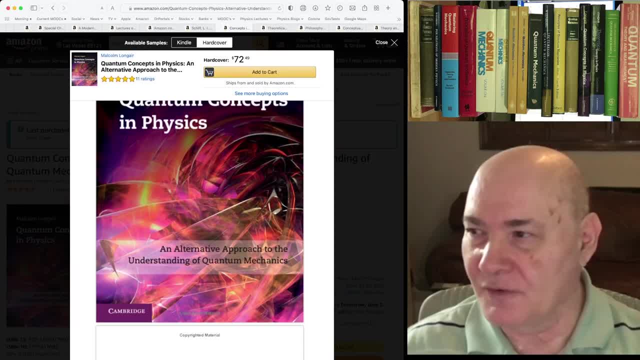 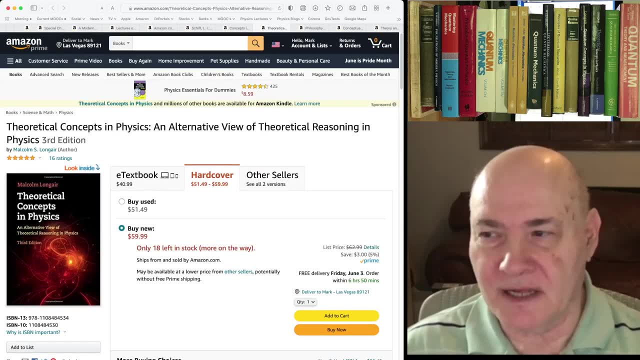 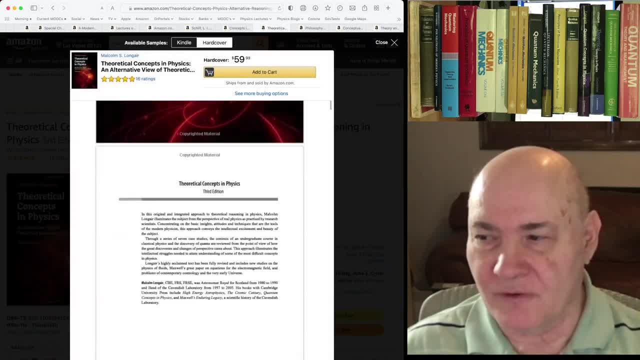 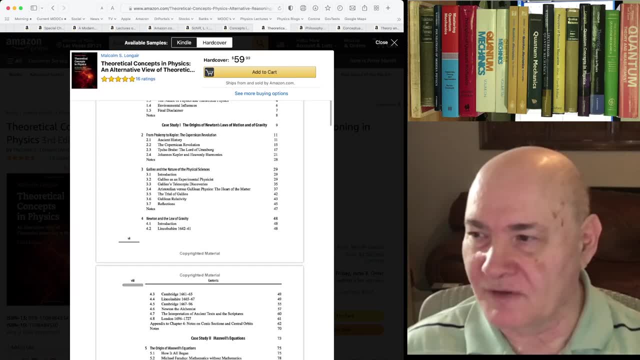 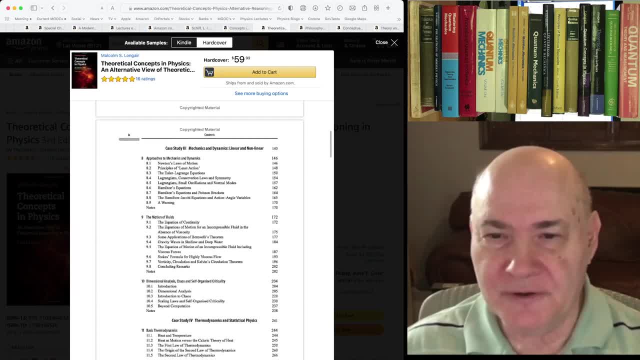 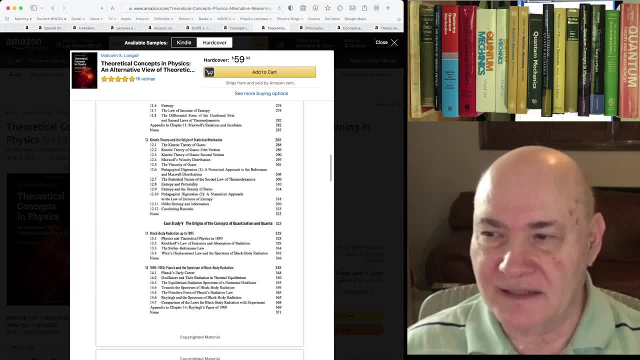 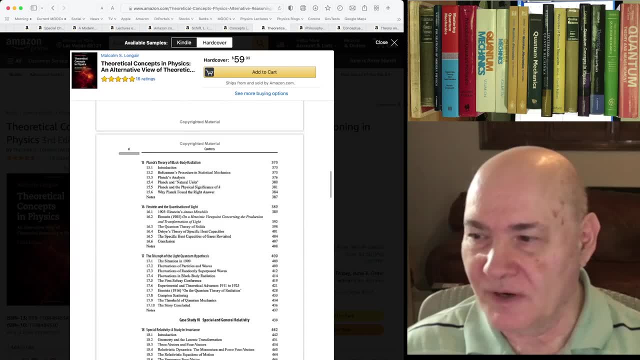 in statistical physics. if you want to see how Planck got the Black Body Law and how he guessed and interpolated, it's all here. and then quantization and quanta. Like I said, a lot of this chapter and the previous chapter are in the other book on. 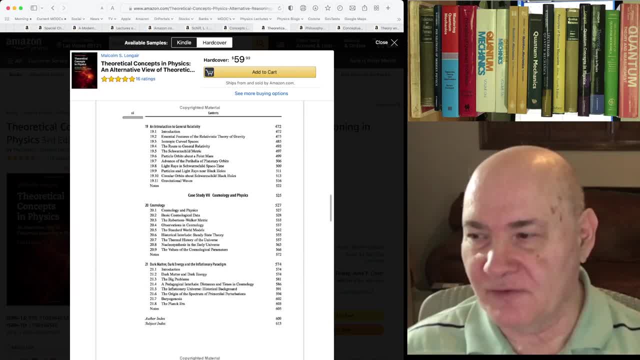 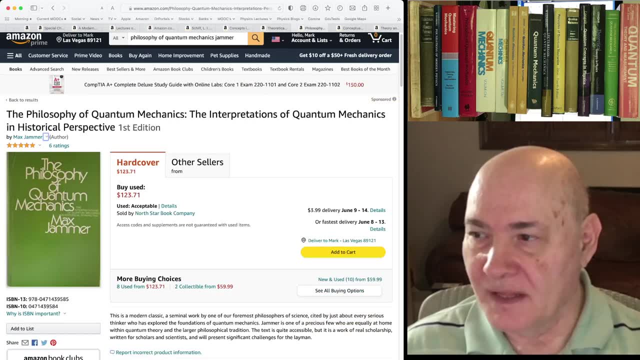 quantum concepts, But also he has sections on special and general relativity and cosmology and particle physics. so I highly recommend both of his books. This is an old book but a classic book: The Philosophy of Quantum Mechanics by Max Jammer. Today there are many books on philosophy of quantum. 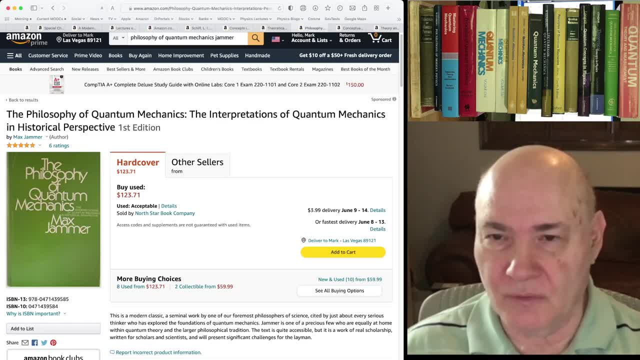 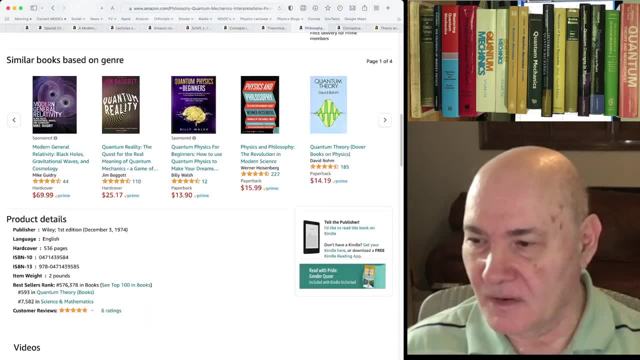 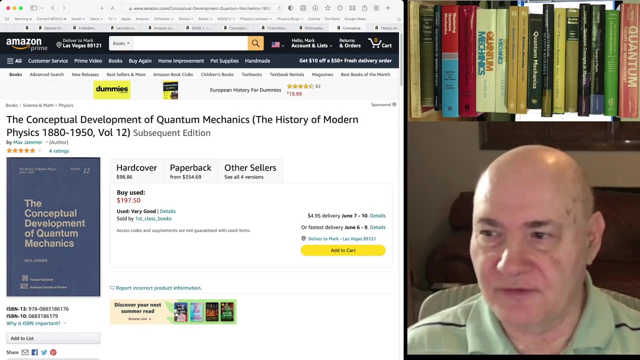 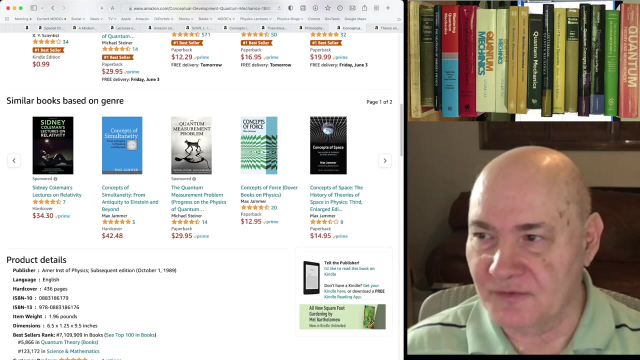 mechanics, but I think this one is still worth worthwhile reading. and also look at some of the other books on quantum mechanics and philosophy. Jammer also wrote a classic study on the conceptual development of quantum mechanics and I remember going to the library to read this. and the thing is: 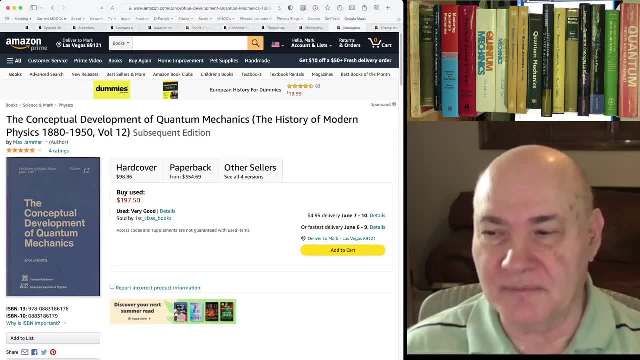 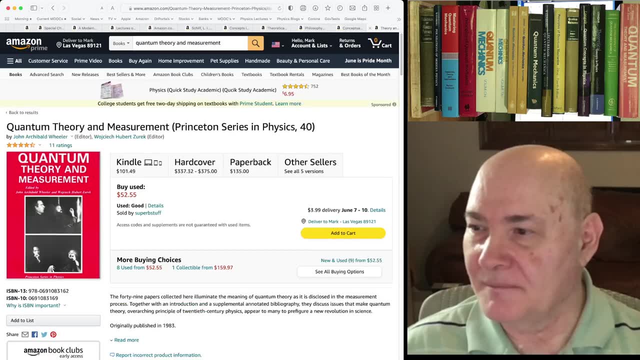 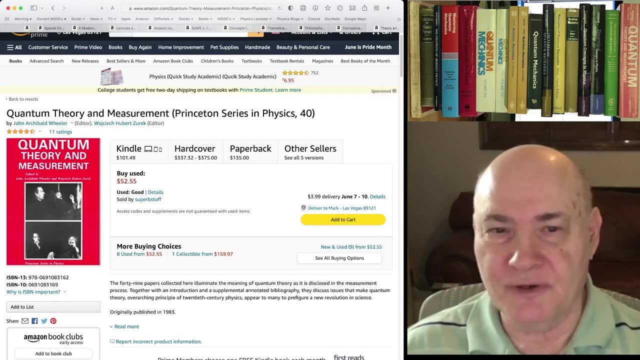 you already have to know quantum mechanics to benefit from this book, But if you read a quantum mechanics textbook, you can read this and profit. And then, finally, my last book. I remember reading a book on Quantum Theory and Measurement. I'll have a lot more books on this, I think on the 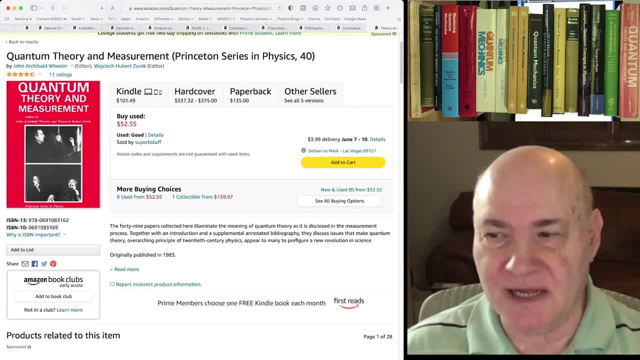 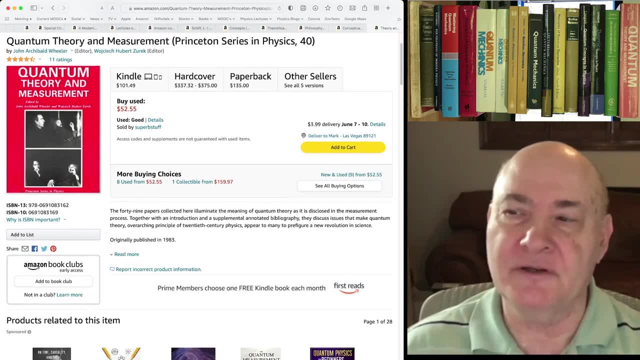 playlist. but this is sort of like a reprint volume—it reprints a lot of the early human data papers. it was written, published in the early 80s and it's a good idea, good place to start if you're interested in the whole thing on quantum theory and 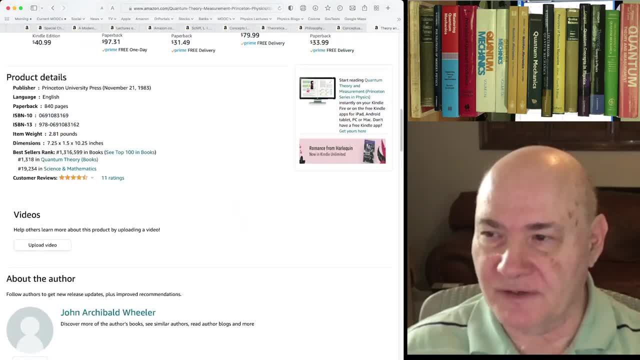 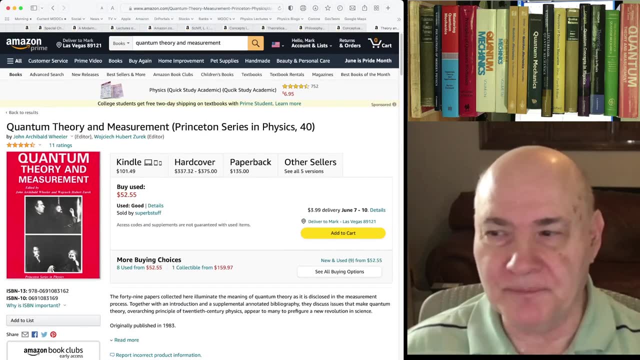 measurement and the philosophy of quantum mechanics. so it's very expensive. try and get some kind of used edition, because somehow Princeton is like reprinting it and charging a fortune. but so those are the books I recommend on quantum mechanics, and there are many, many, many more that I've left out. 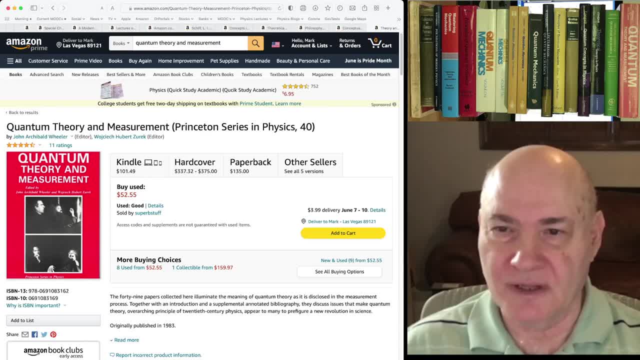 there are some that are more advanced, some that are less advanced. these are probably the major ones that are that I own, that I happen to own and that are also sometimes you a lot often used in American classrooms. but it's you need to own about two or three quantum mechanics books, maybe even more, to get a real good. 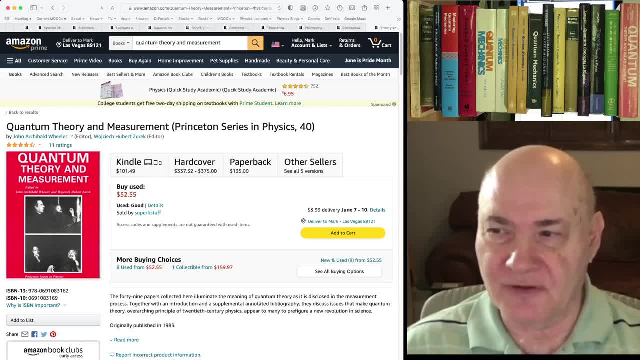 understanding of the subject and right now, like I said, my number one recommendation is start with Barton Mastering Quantum Mechanics, and then maybe go to Ballantyne and Weinberg on their graduate level quantum mechanics books. so thank you very much for watching and I'll be back next time updating the playlist on advanced classical mechanics. 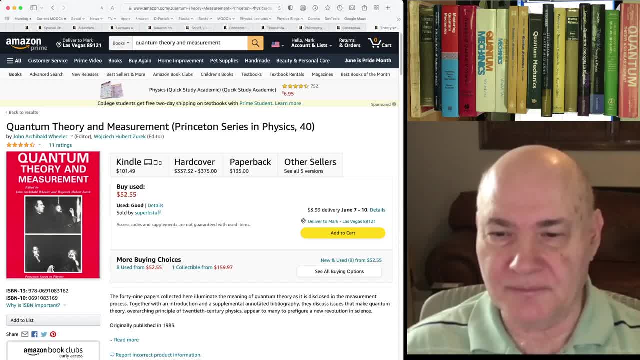 and classical electromagnetism. thank you very much.